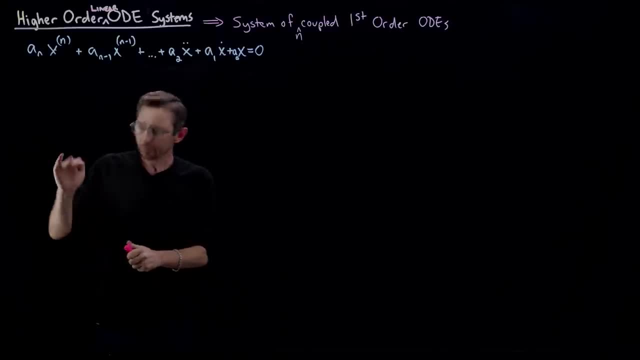 I think you're going to love it. Okay, So what we're trying to do is take this high order system and write it as a matrix system of first order equations, And we can do that pretty simply by introducing new variables. So we introduce: introduce new variables. 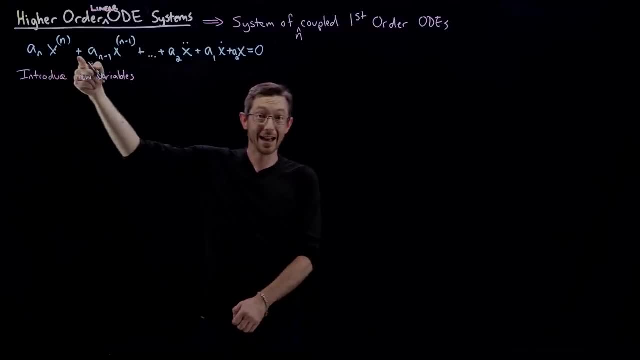 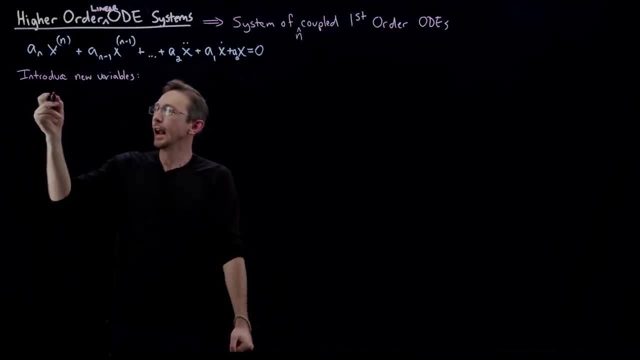 So currently the only variable we have here is X, And now we're going to introduce some new variables. I actually opened up a new pack of markers because I'm so excited about this lecture, And so we're going to say our first variable is just our original state, x. Our second variable is going to be x- dot. 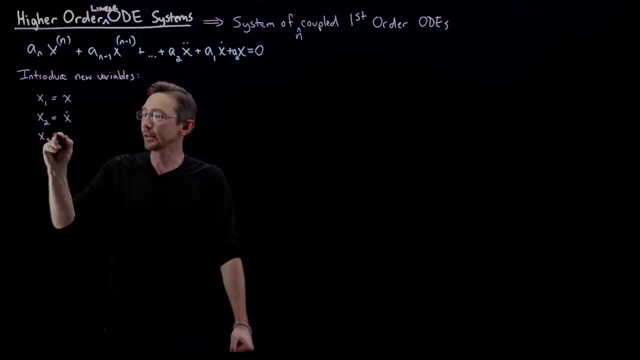 the first derivative of x, x3 is going to be x double dot. You see the pattern here All the way down. I'm going to have n of these variables, So I have an nth order differential equation, And so I'm going to write this in terms of n coupled first order equations in these new 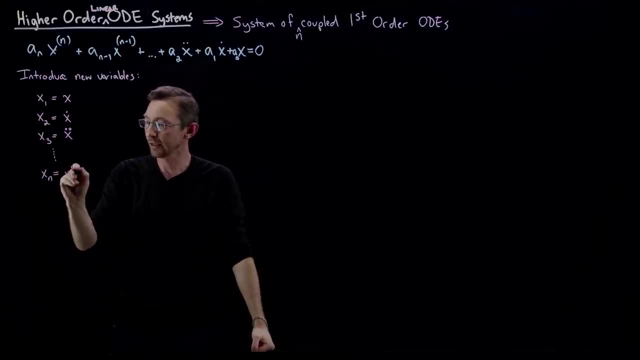 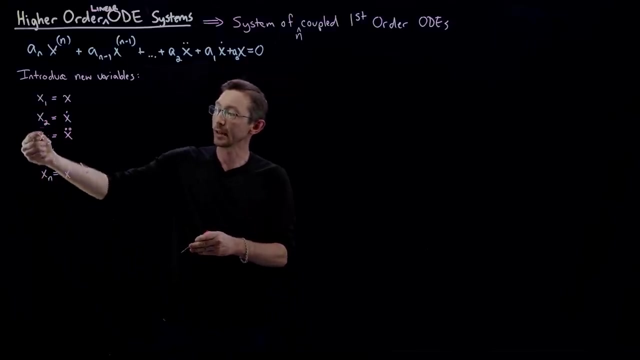 variables, where my last one is the n minus 1th derivative: the n minus 1th derivative. Okay, so this is my new state vector. that I'm going to be dealing with is this: x1 through xn, where each state in this vector represents the state. my original variable x and all of its. 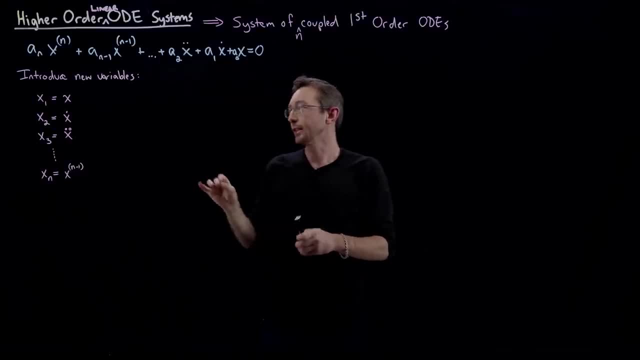 derivatives up to n minus 1.. And so, specifically, I can write down a pretty simple differential equation or something like that, and I can write down a pretty simple differential equation or something like that. and I can write down a pretty simple differential equation or something. 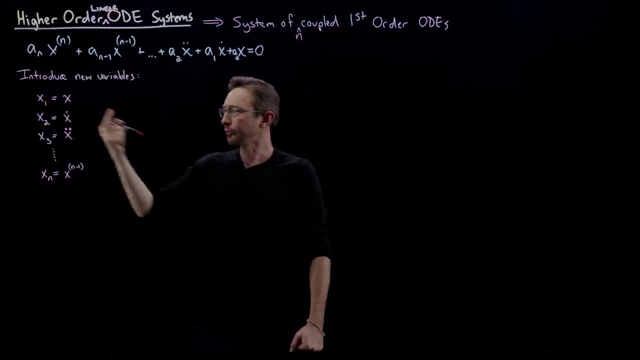 of differential equations. So what we're going to write down is, of course, x1 dot. x1 dot is literally just x dot and x dot is x2.. So we say x1 dot equals x2.. I'm going to repeat. 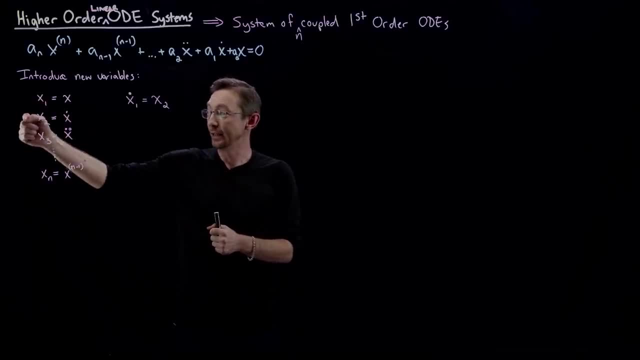 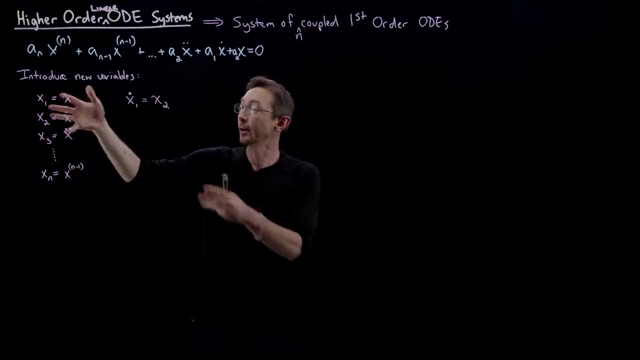 this one time, very important- We're going to take the DDT of each of these variables. We're going to take the DDT of each of these variables. We're going to take the DDT of each of these variables And then we're going to represent those in terms of x1, x2, x3, and so on and so forth. We want a. 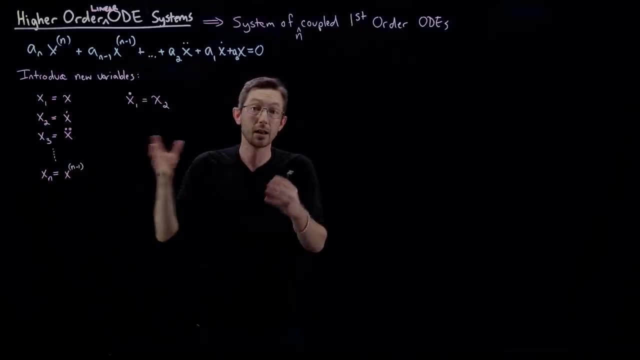 closed form system of the derivatives of all of these states as a linear combination of those n states. So I start with x1, and I compute x1 dot. x1 dot is the time derivative of x. you know x dot, which is my second state, x2.. So x1 dot equals x2.. Similarly, x2 dot. if I have x2 dot, that's x dot. 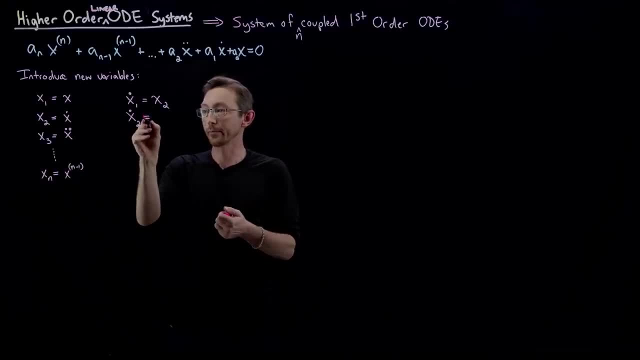 dot, or x double dot, which is my state, x3. And so on and so forth. So xk is going to be the DDT of xk is going to be xk plus 1. And that works all the way for all of these rows, until the very last. 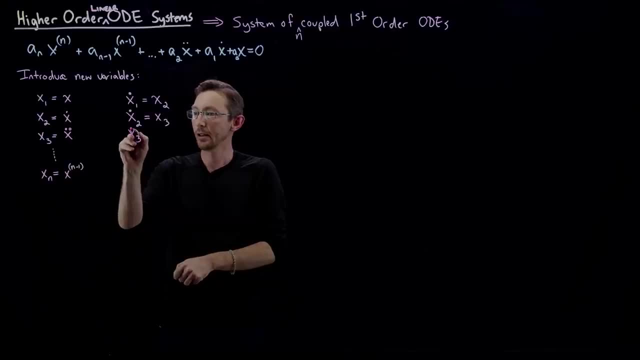 one. So let's say x3 dot is going to be x double dot, another dot, So the DDT of this x double dot is now x triple dot, which is going to be my x4 state, So x4, and so on and so forth, until this very last row equation where now I'm going to have xn dot. 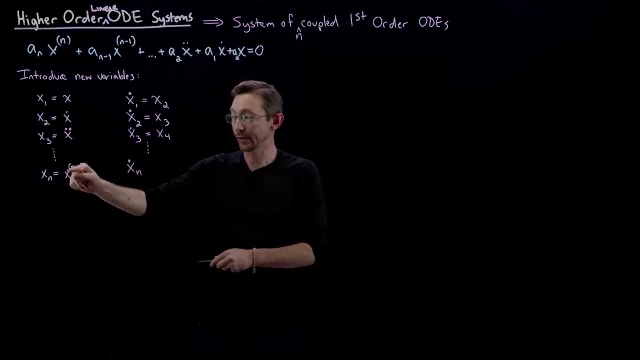 The time derivative of this state is the time derivative of this. And if we add one more derivative to the n minus 1th derivative, we get the x to the nth derivative. This equals, you know, the nth derivative of x, which is: 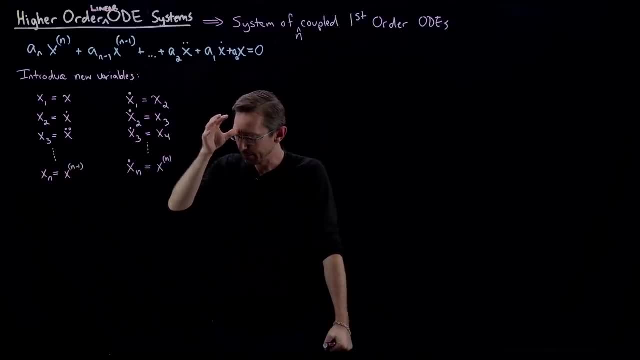 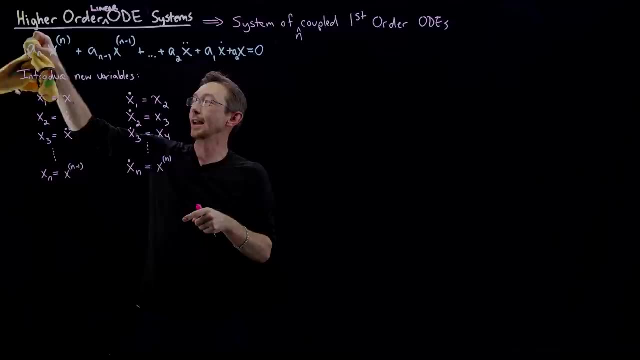 space Specifically. can I just make my life easier for one moment? Please bear with me. I'm going to divide all of these coefficients by an. That's totally fine, because I can divide all of my coefficients by an, And these are just. 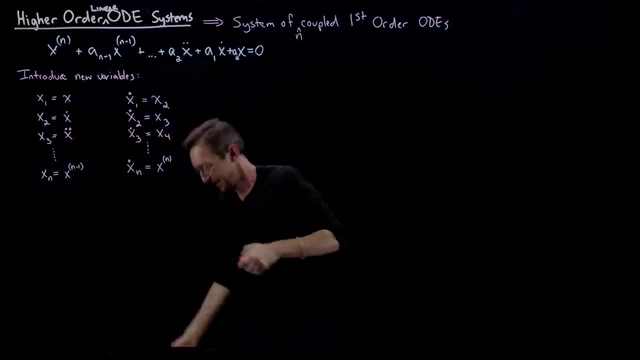 new coefficients and it still equals 0.. I'm going to get rid of that here real quick, And so now what I'm trying to do. this last row, equation, xn dot, which is the nth derivative. it equals all of this stuff. 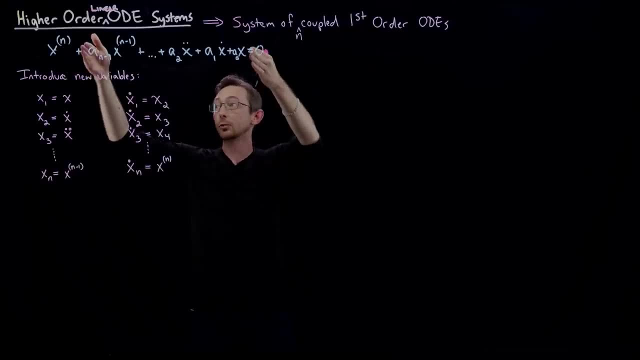 moved over to the right hand side. the nth derivative equals minus all of this stuff here. so this literally equals, this equals. I'm just gonna do it. it's minus all of this stuff, minus a naught X, minus a 1. so X is just X 1, so minus a naught X. 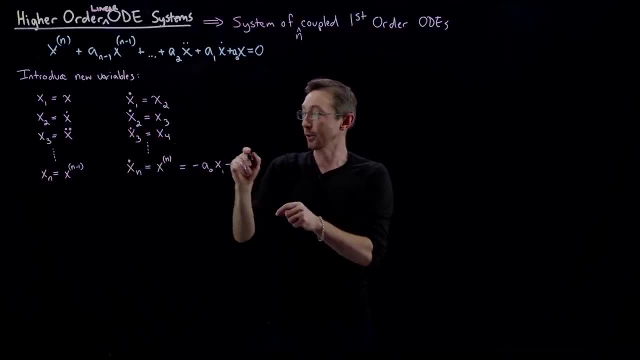 1 minus a 1. X dot, which is X, which is X. 2 minus a 1. X 2 minus a 2. second derivative is X 3. I just want to be very careful: minus, dot, dot, dot, dot dot minus a n, minus 1 times the n minus 1. th derivative, which is my X n. 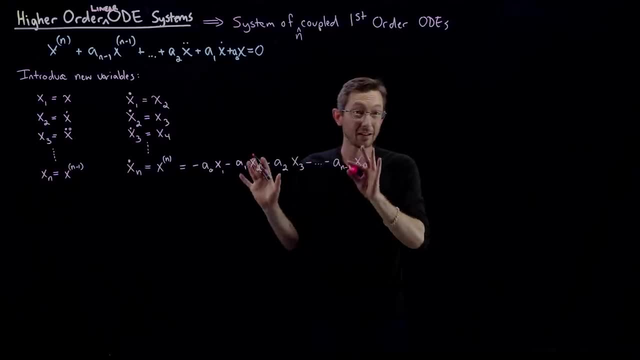 okay, I think this is correct. I'm gonna just look at my notes. that looks like I got it right and there's minuses on all of these. okay, so I'm not completely convinced that at this point. maybe you shouldn't be completely convinced at this point that I've actually 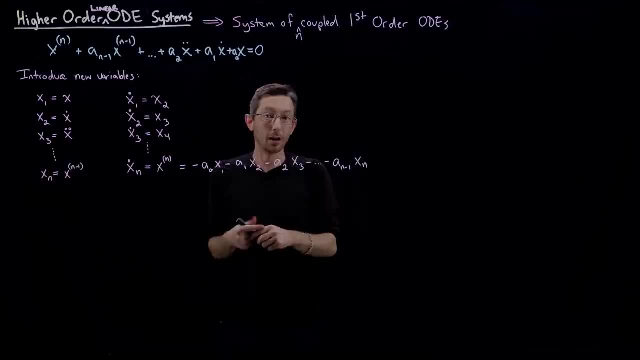 done anything to simplify my system, but very soon I will hopefully convince you that this is actually much, much easier to work with. so what I'm gonna do now- and I think I'll switch to to blue here- is now: what we're going to do is we're going to be able to write this, all this whole system. 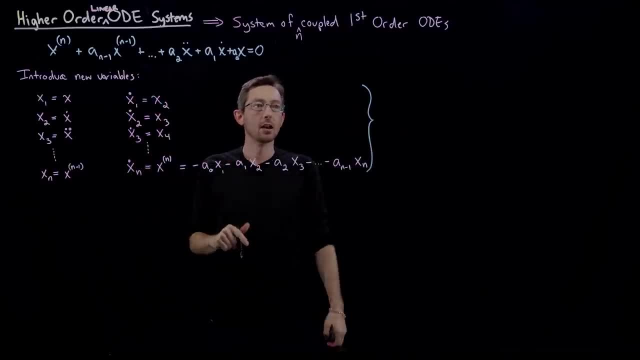 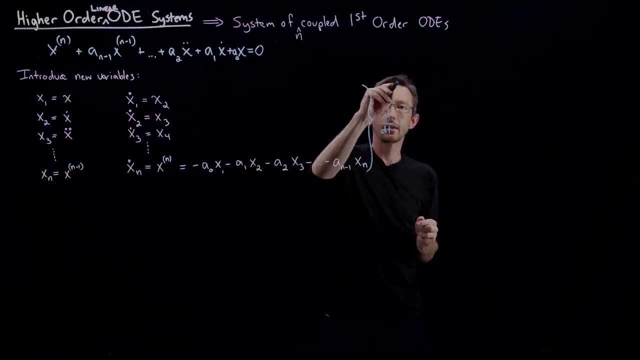 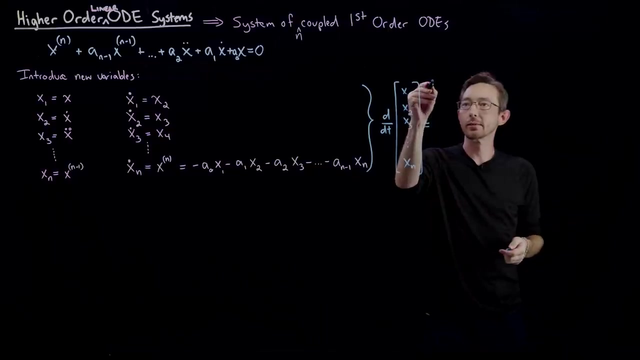 of equations. I want to make sure I have enough space here. I can write this as ddt of my vector: X 1, X 2, X 3, dot, dot, dot all the way to X n. this is going to be a big matrix and I want to make sure to give myself space here, so I'll go all the way up to the end. 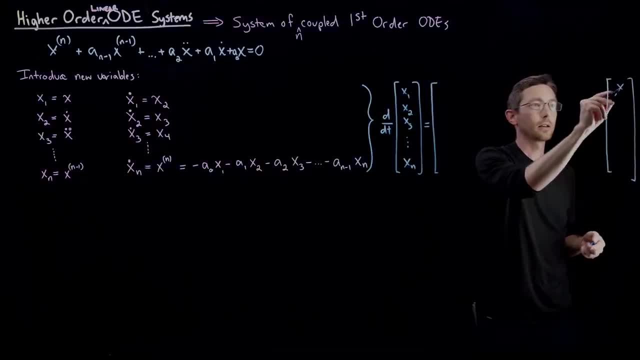 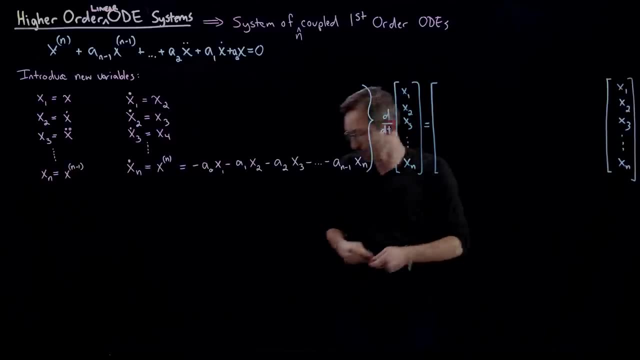 a big matrix times: X, 1, X, 2, X, 3, dot, dot, dot, X n. okay, and I don't want to be sloppy here- X n, X n, X n, X, 3, dot, dot, dot, all the way to X n. okay, and so this is really easy to read off what the 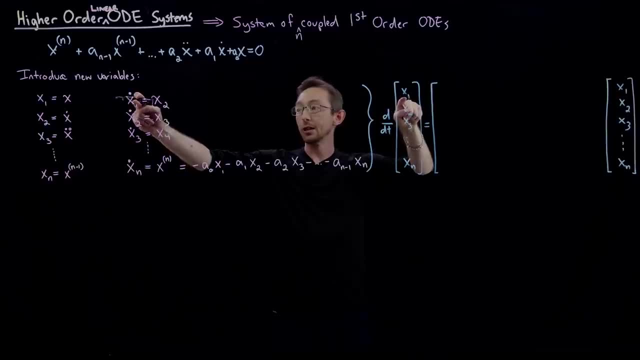 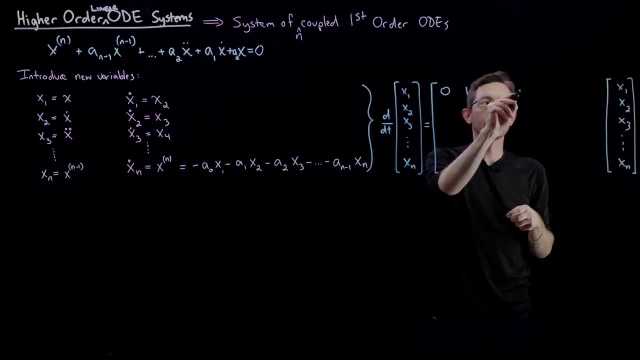 terms of this big matrix are X 1. dot equals X 2, so that is 0, 1, 0, dot, dot, dot. you know. what I'm going to do here is I'm going to add one more, one more row. should I add one more row for the X n minus 1? I think I'm going to. I think you're going to thank me later. 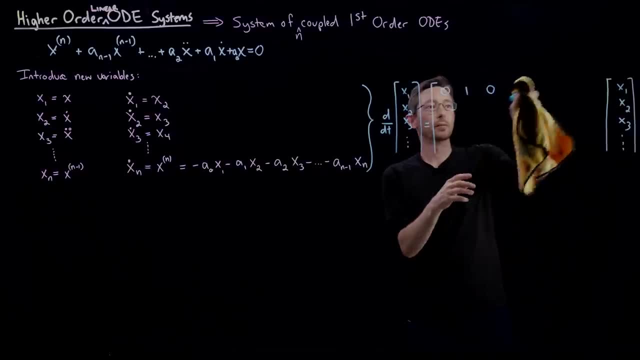 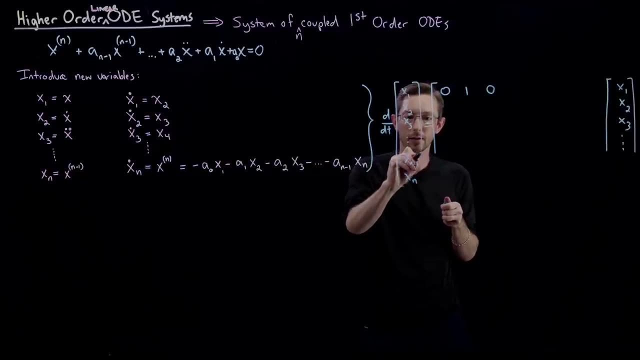 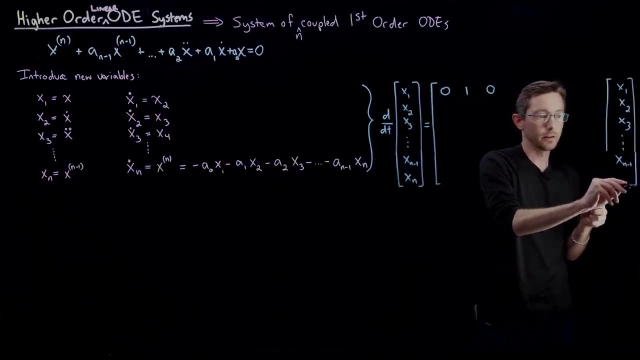 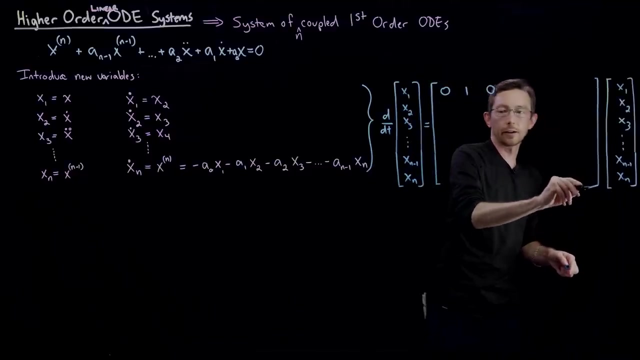 if I add one more row for X n minus 1, I'll make this a little bit more concise. so X n minus 1, X n. okay, this is going to go down to X n minus 1, to X n. good, and now this big matrix here, okay, so, 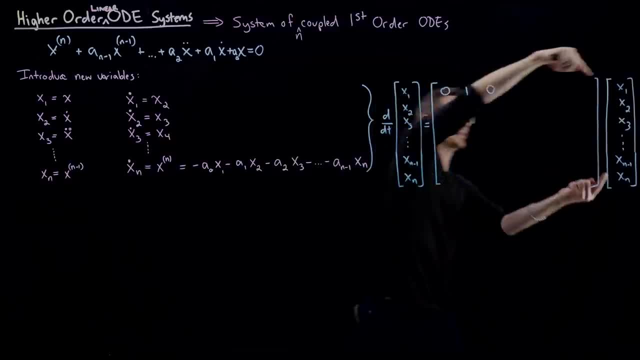 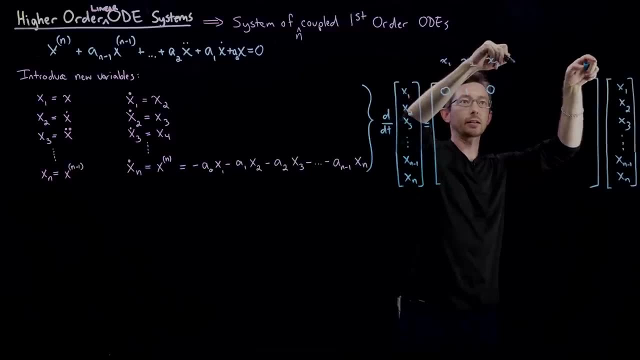 the X 1 dot term is X 2, which if I take this and I multiply it over, this is kind of the, you know, the x1 spot, the x2 spot, the x3 spot, dot, dot, dot, xn minus 1 spot, xn spot. 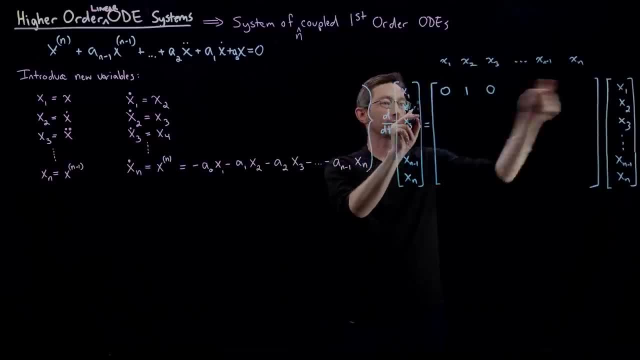 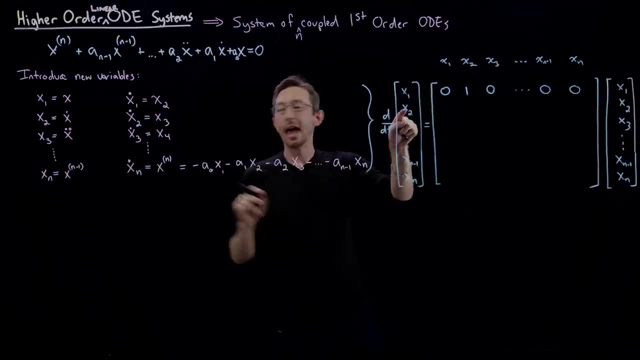 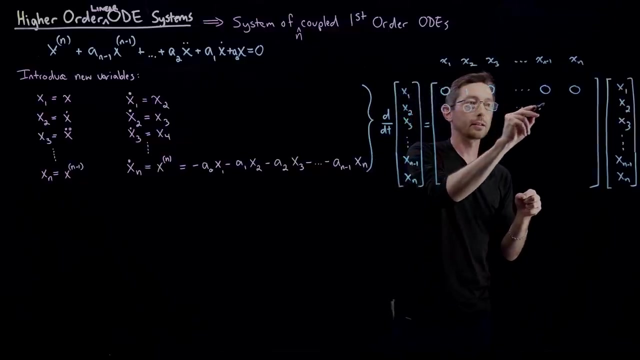 if I multiply this whole thing over, So x1 dot equals x2,, so that's 0, 1, 0, dot, dot, dot, 0, 0.. Easy, easy, easy. x2, dot is x3,, so similarly, that is 0, 0, 1, dot, dot, dot. 0 is everywhere else. 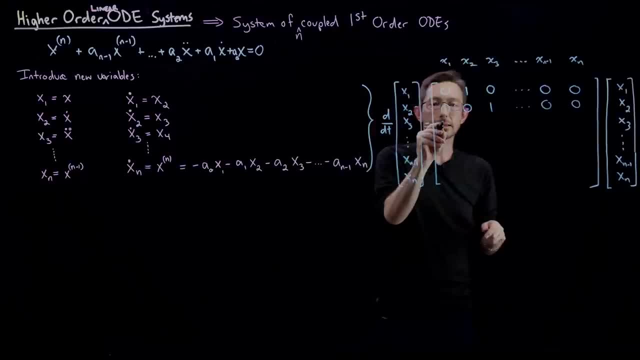 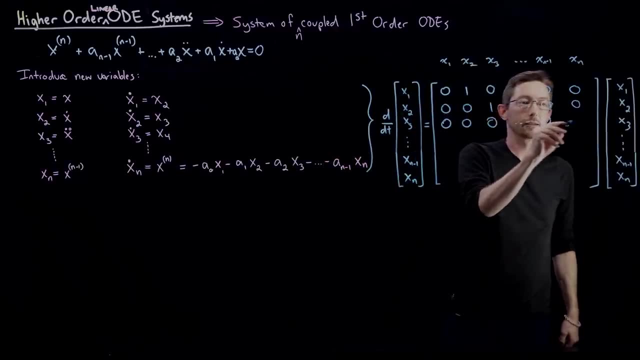 The x3 dot is x4, which is you know, 0, 0, 0,. the next column would have a 1 in it, but I don't have it written here. dot, dot, dot, 0, 0.. 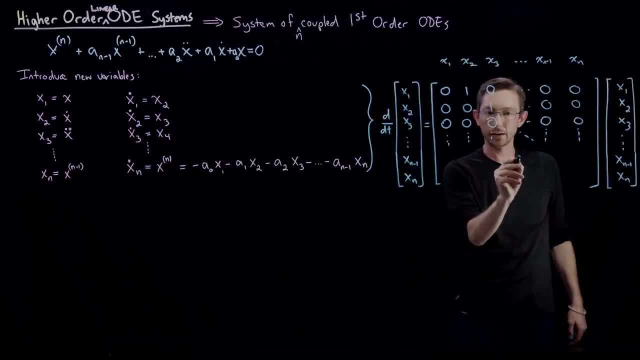 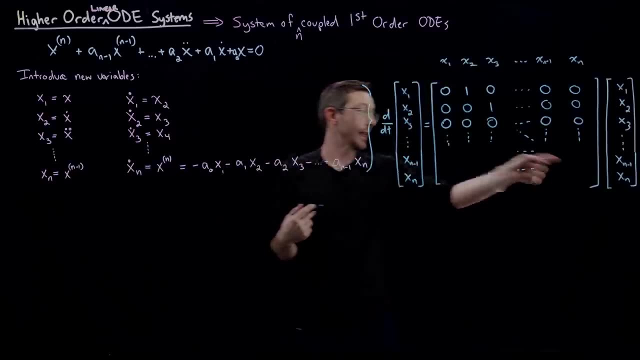 Okay, let's just not mess anything up here. And now the xn minus 1th derivative: ddt of this is xn, so I'm going to have zeros everywhere here, up until the very last derivative. So ddt of xn minus 1 should be xn, and that is in fact what I get if I multiply this. 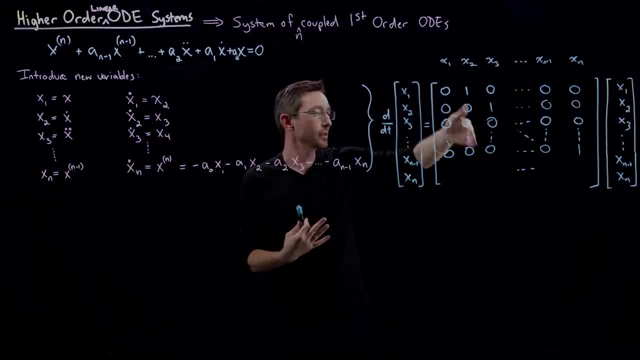 So so far, most of this matrix is almost trivial. It's mostly zeros and it has one diagonal of 1s saying that x1 dot equals x2, x2 dot equals x3, x3 dot equals x4, dot, dot, dot, dot dot. 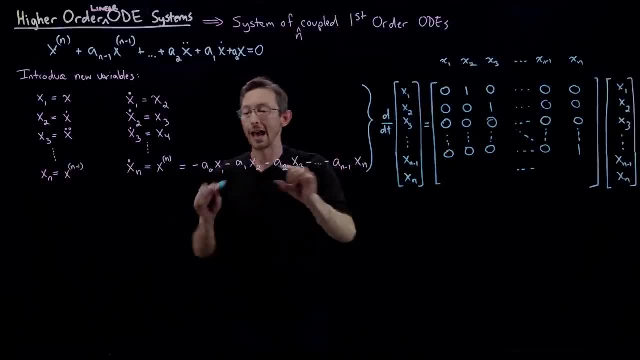 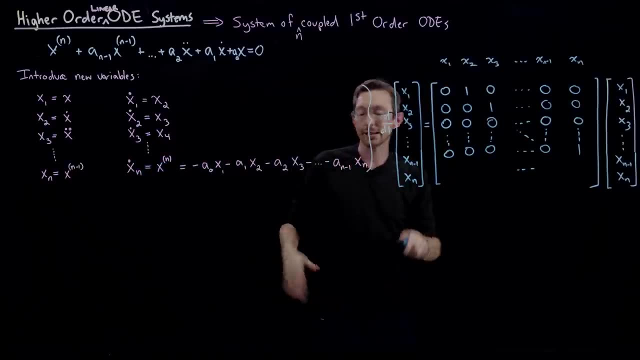 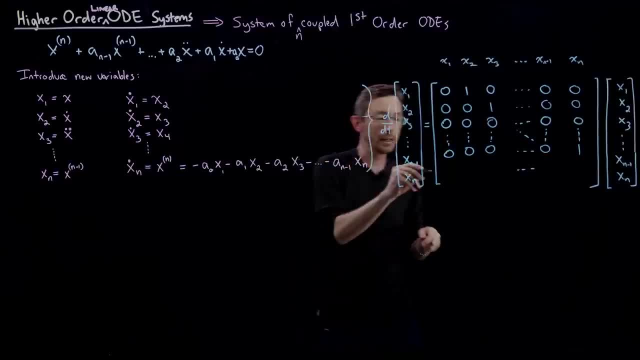 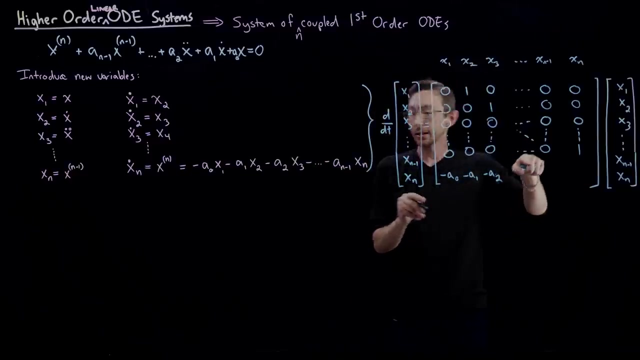 xn dot is minus a0 in the x1, minus a1, x2, minus a3, no a2, sorry, I really should be careful here. minus a2 times x3, dot, dot, dot, dot, dot minus a. 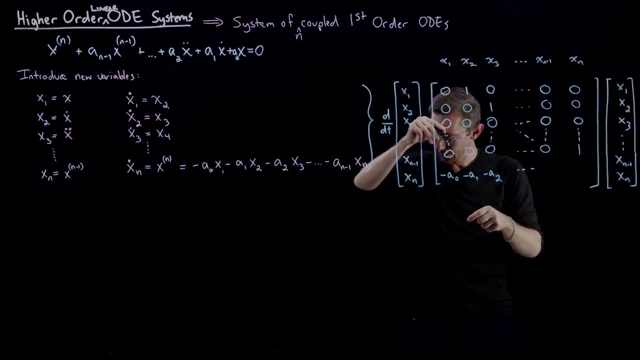 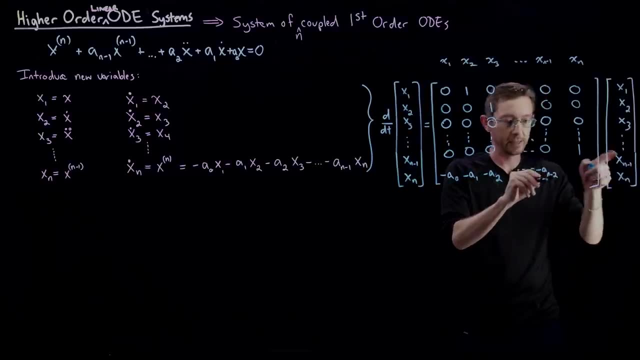 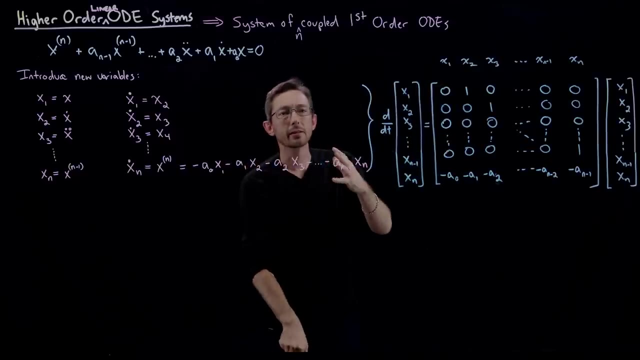 n minus 1,. yeah, minus a n minus 2 times xn minus 1, and minus a n minus 1 times xn. So you can kind of convince yourself. just go through the motions. you know, take this vector. 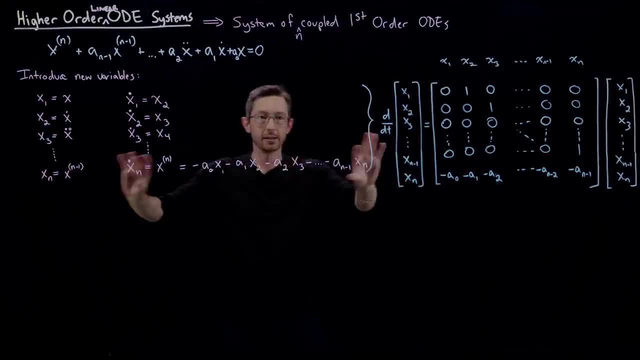 knock it on its side, multiply it by this and convince yourself that that's equal to this equation here, And in fact all of these equations are represented by this matrix system of equations. So now this is actually something that we can really work with. This is linear algebra. 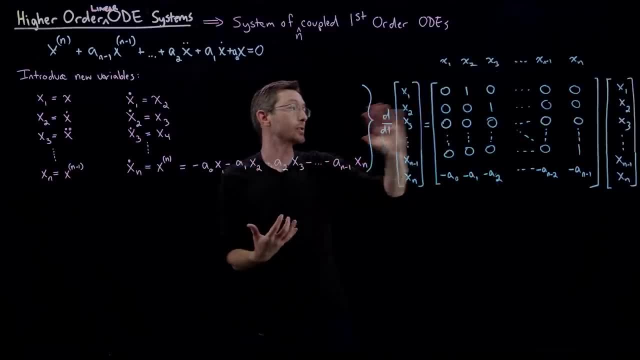 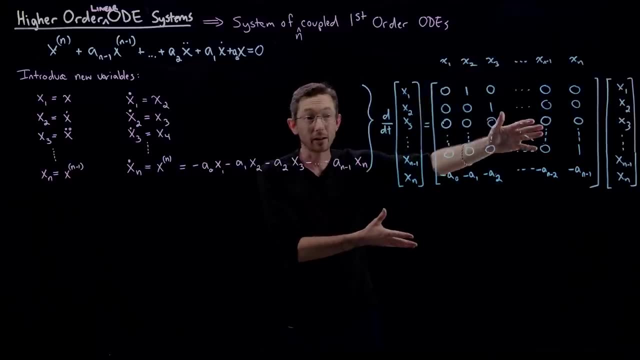 We can. I'm going to show you in the next few lectures. we can solve this system in closed form by finding the eigenvalues and eigenvectors of this matrix. We can integrate this numerically way, way easier than working with this object here Finding, even if I wanted to find- the 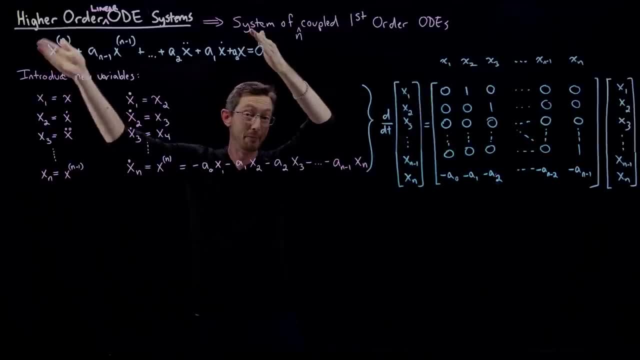 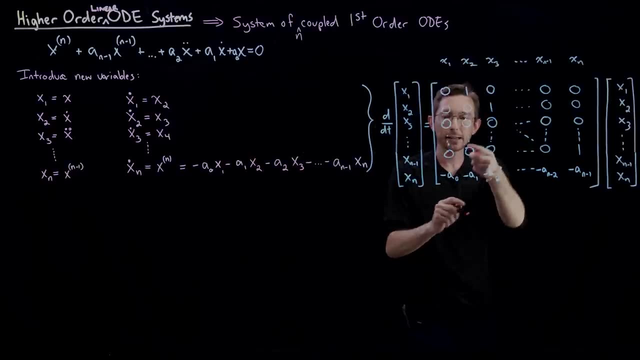 characteristic, the roots of the characteristic polynomial. the best way to do that is to find the eigenvalues of this A matrix which I'll show you in a minute, And then we can solve this system in a minute. So I'll just write this and kind of summarize this whole thing here You can write: 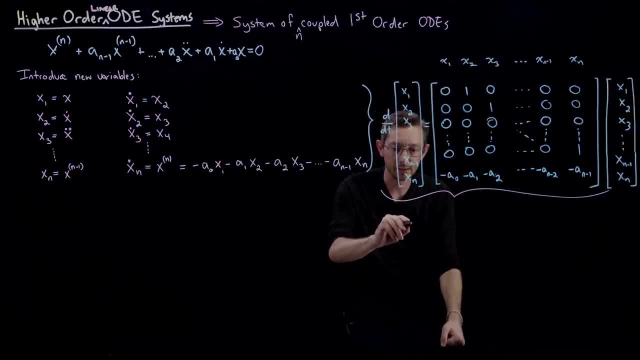 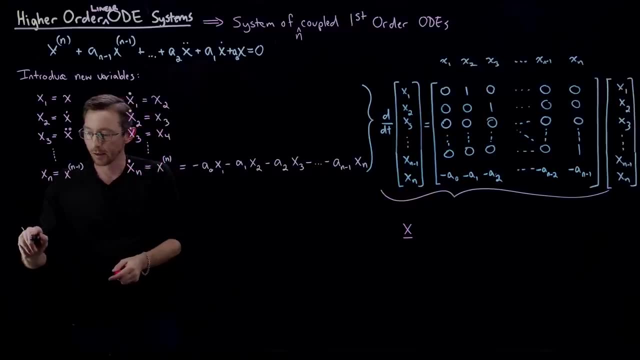 as a big vector. x. This is, you know, I'm going to use the notation- that an underbar means that this is a big vector of states x. This is literally underbar. x equals, you know, x1,, x2,, x3,. 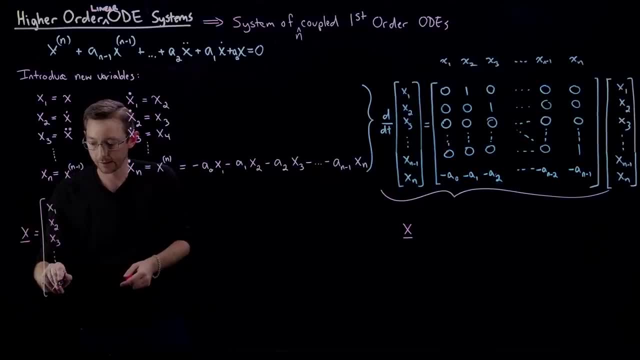 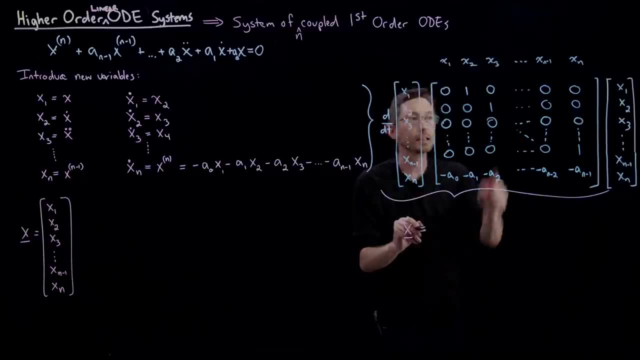 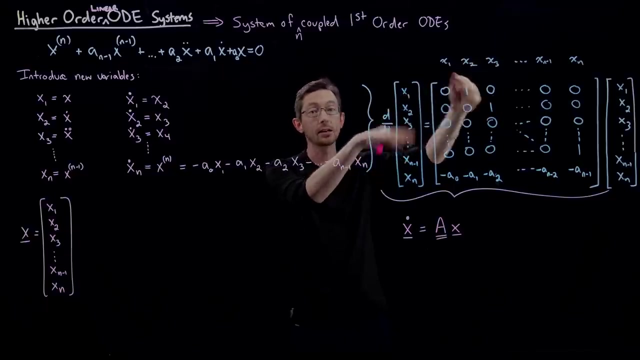 dot, dot, dot xn minus 1, xn. That's what this underbar means. And so this x vector dot is equal to this big A matrix, this big A matrix times x. So this is a matrix system of equations. They are coupled because x1 depends on x2 and x2 depends on x3. 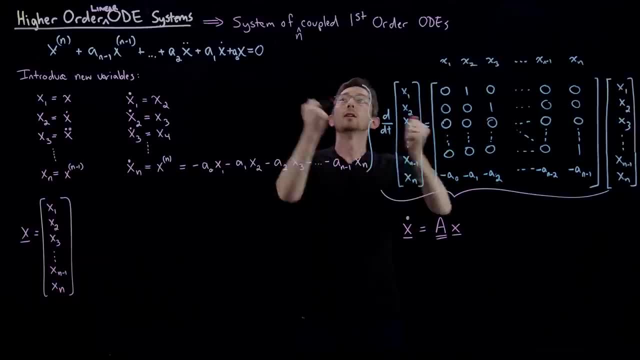 and dot, dot, dot and xn depends on all of them. So it's coupled. It's coupled. There are n coupled first order equations, because I'm only taking a single time. derivative of any of these states. Now, of course, morally, we know that these states represent higher derivatives of my original. 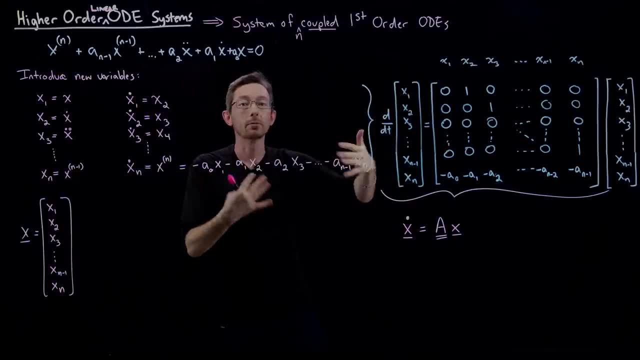 variable x. But here we have transformed the system so it's simpler. So I'm only dealing with first derivatives of a larger dimensional, a larger state, x, you know underbar- that has n components. This is a vector, This is a matrix A And this is another vector. 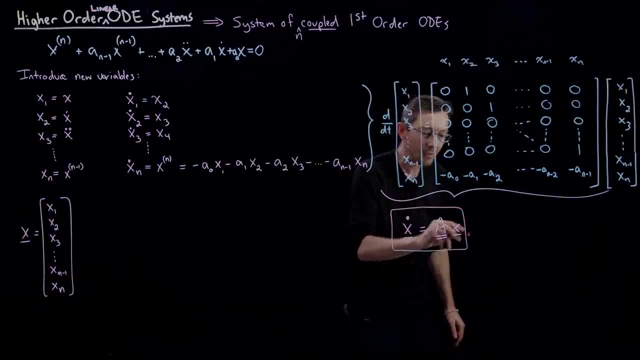 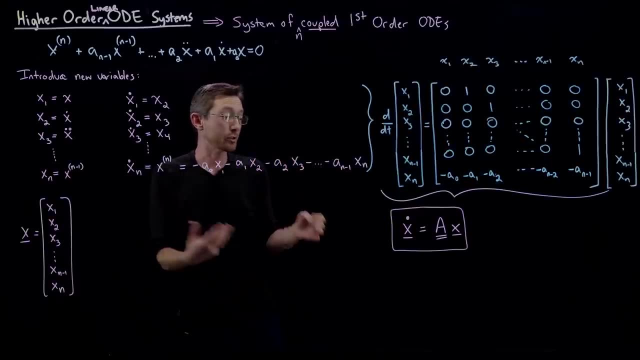 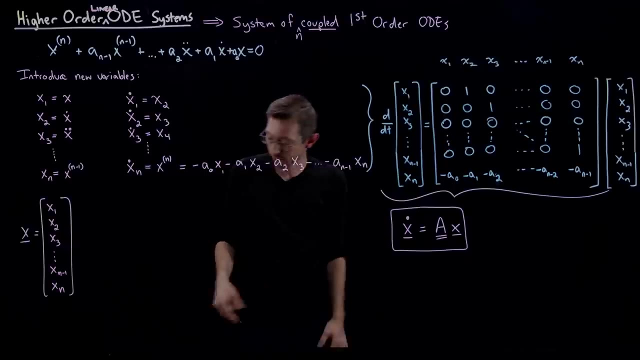 So this is a huge deal, This. we are going to spend most of the next- I would say four lectures, maybe five or six lectures- now dealing with this matrix system of equations, because this is where linear algebra and differential equations meet. So this is where 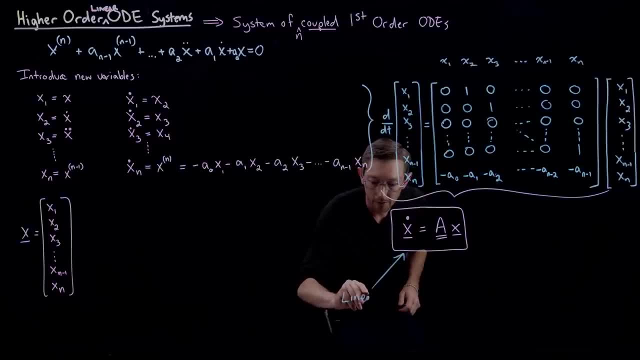 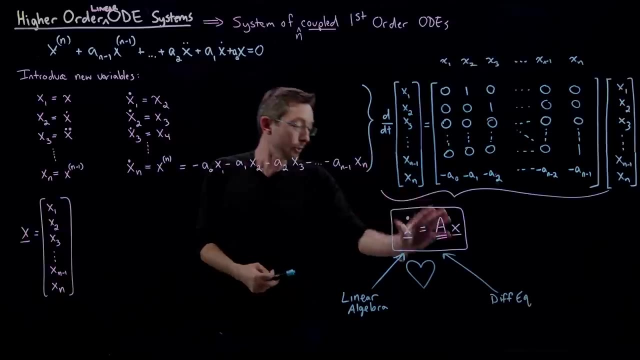 you know linear algebra, linear algebra and differential equations, diff EQ. this is where they meet And it is wonderful. Okay, matrix system of equations is where we're going to use all of our powerful techniques from linear algebra to solve really, really interesting systems in. 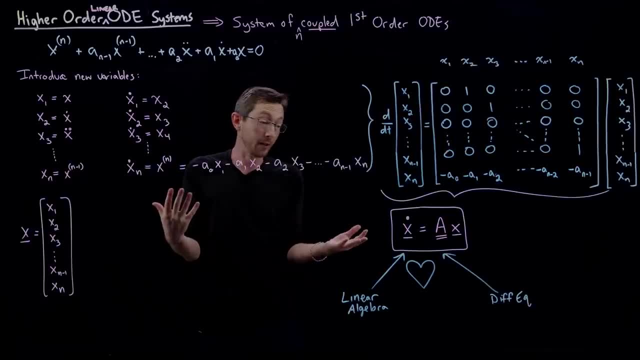 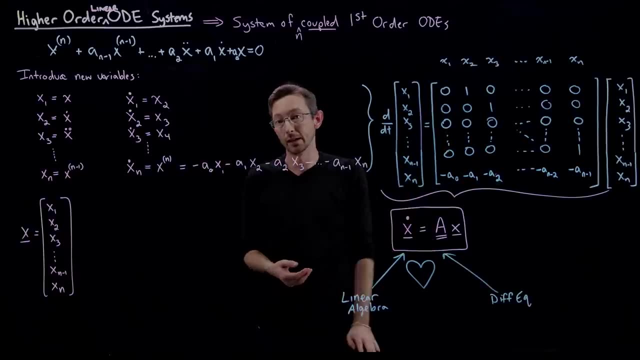 differential equations- and for me, this is the high watermark you know of applied math- really is when we start analyzing these systems and understanding the real world in terms of both linear algebra and differential equations. okay, good, that's. the main thing I wanted to show you is how you can take any higher. 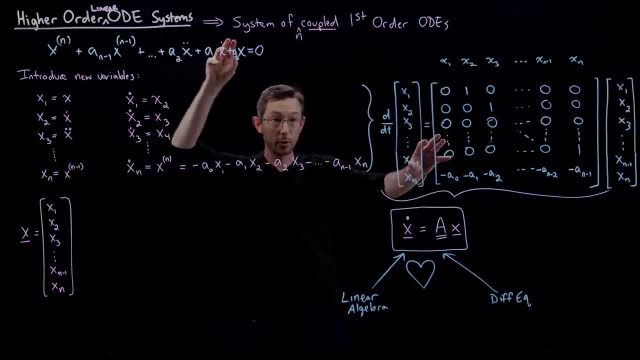 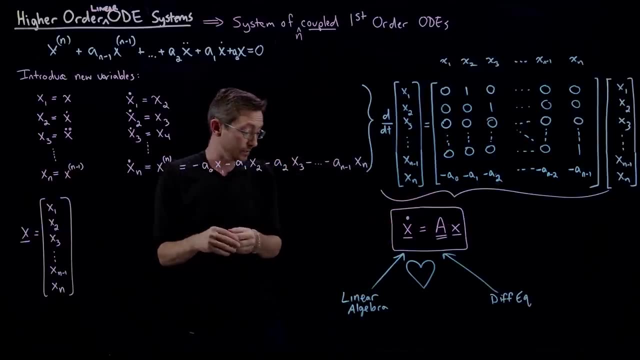 order system and turn it into a coupled system of first-order equations, which gives you this matrix system of equations. what I think I'm going to show you for the rest of this lecture, because I do have a little bit of time, is the next thing I'm going to show you. this is very important- is that the eigenvalues. 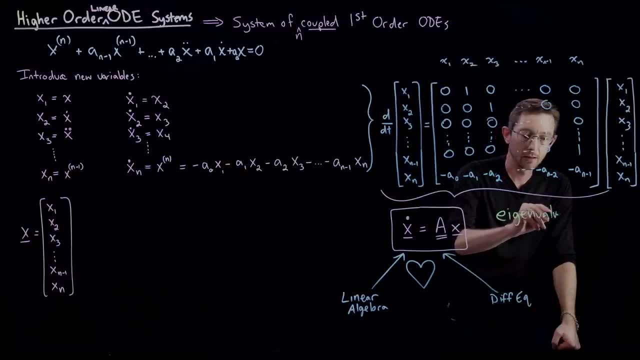 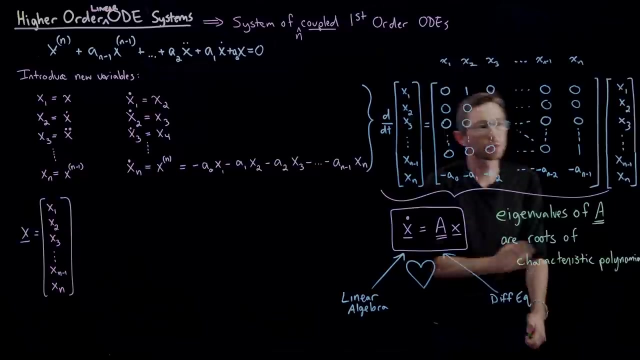 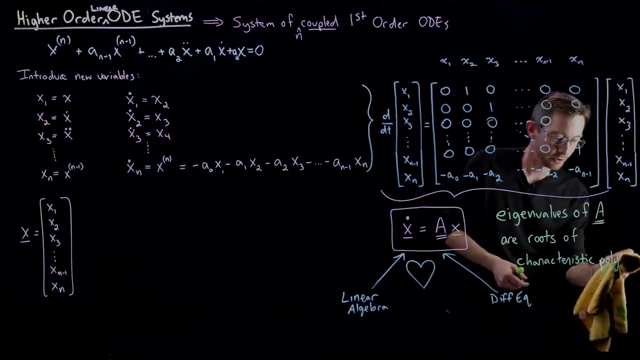 the eigenvalues of a. this, a matrix, are the roots of the characteristic polynomials, are their roots of the characteristic polynomial, and these mean the same thing essentially. I've shown you before that this is true polynomial. sorry, I got got cut off. these are the roots of the characteristic polynomial. let's just call it poly, for. 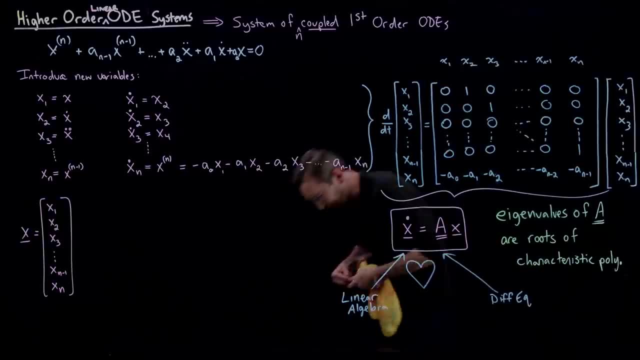 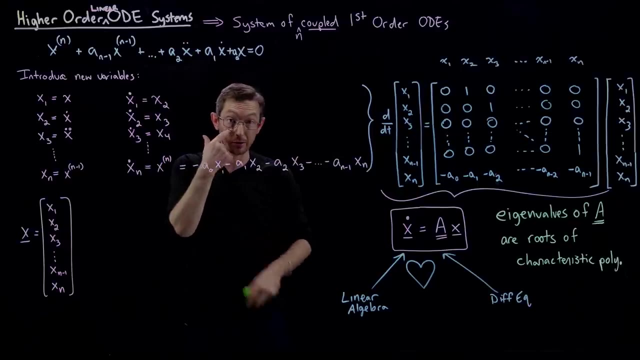 short, we're friends- poly polynomial, and I've shown you this for a second order system before, and so now I'm just gonna you know again, convince you that the eigenvalues of this, a matrix are the roots of the characteristic polynomial. a matrix are equivalent to the roots of this characteristic polynomial. okay, so I? 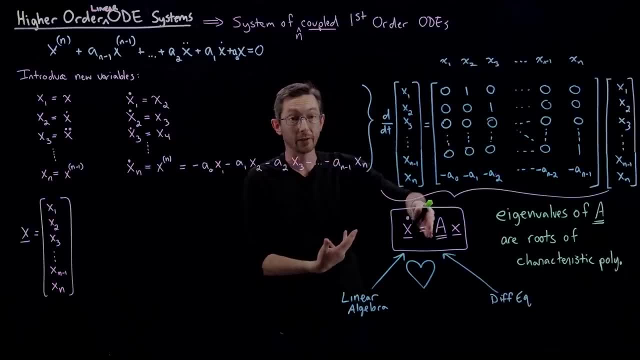 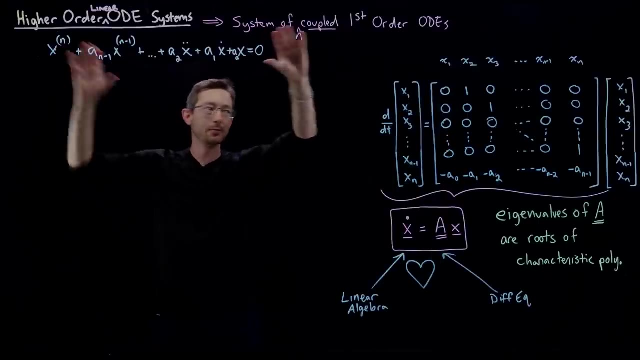 can kind of my eigenvalue equation for how I solve for the eigenvalues of a. that eigenvalue equation is my characteristic polynomial. I'm going to erase this and I'm going to show you that. just stay put, okay. so we have shown how you take this system and, sorry, this high-order ODE. 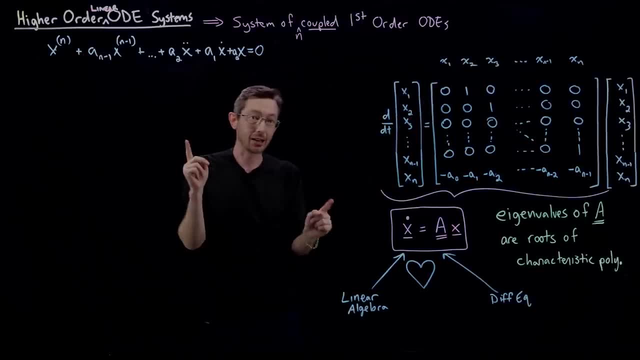 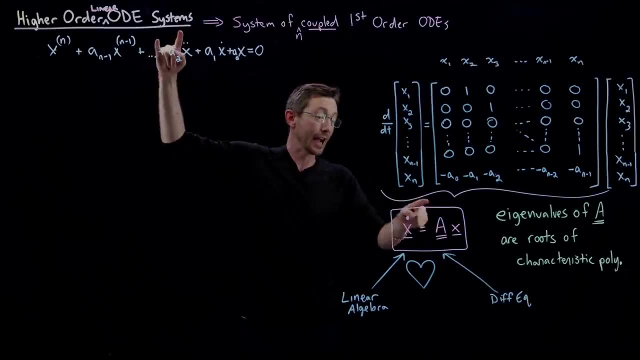 and turn it into a system of first-order ODEs. and I claim that the characteristic polynomial of this equation is the same as the eigenvalue equation for this, a matrix, this big matrix here that relates all of these, these states, and specifically the eigenvalue equation, the equation you use. 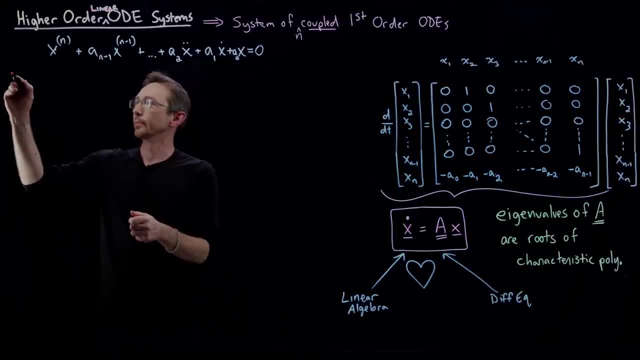 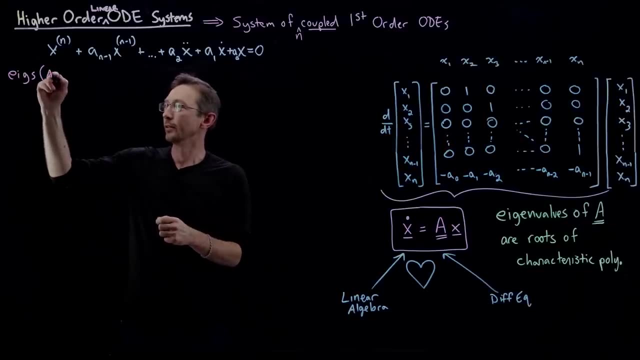 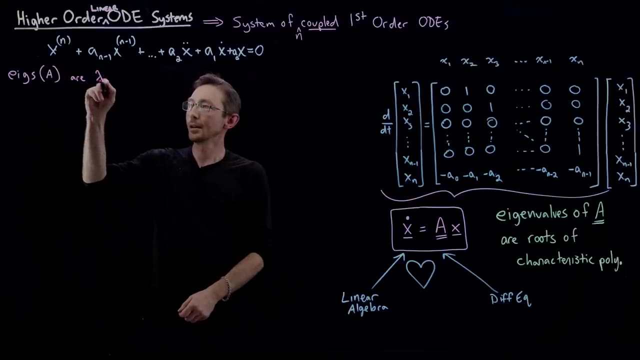 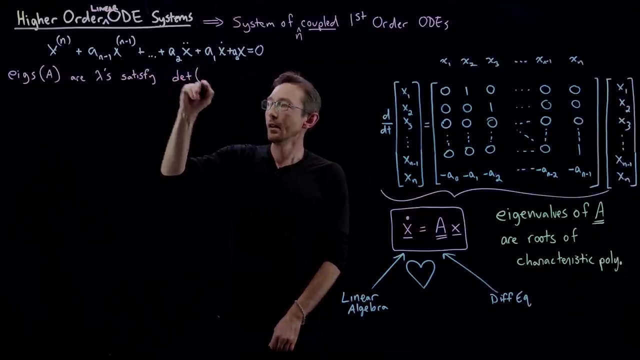 to find the eigenvalues of a. so the let's I'm just going to use for short, we call these the eggs sometime. the eigenvalue and the eggs of a are specifically those lambdas. are lambdas that satisfy this equation determinant of a minus lambda times the identity matrix equals 0. now 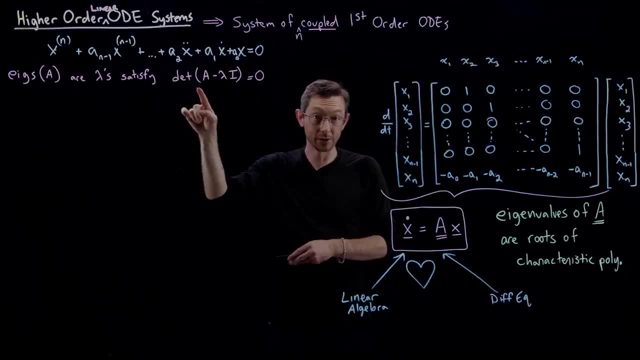 I'm going to derive this from scratch in a couple of lectures very soon, specifically as a: a a set of lambdas that you need to solve this differential equation to solve this differential equation. so if this looks like a bunch of hairy math that came out of nowhere, it is, but I'm going to derive this in a little bit. just take: 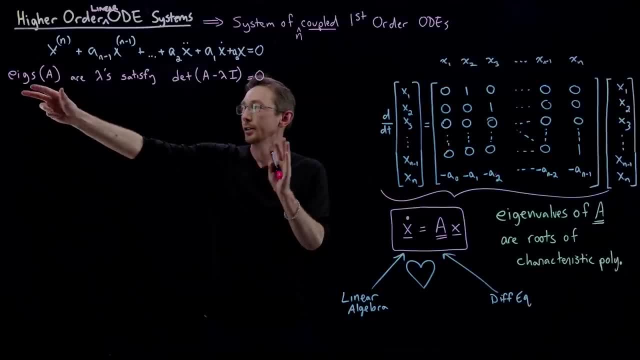 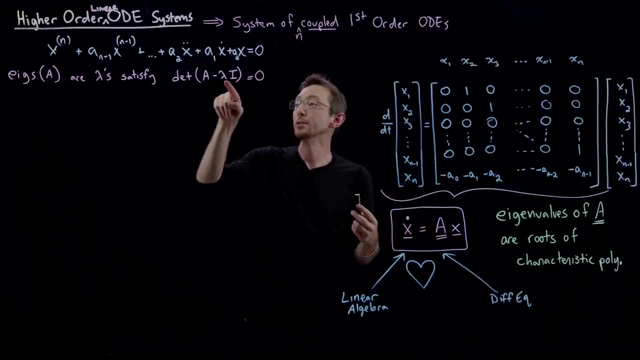 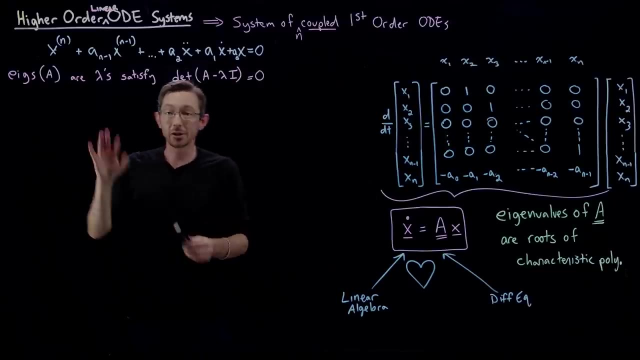 for granted. granted, not granite. take for granted, just for the moment, that this is the expression that you use to solve for eigenvalues of a. okay, this is how you find the eigenvalues of a. is you find the lambdas so that the determinant of this matrix equals 0? okay, and I'm just going to. 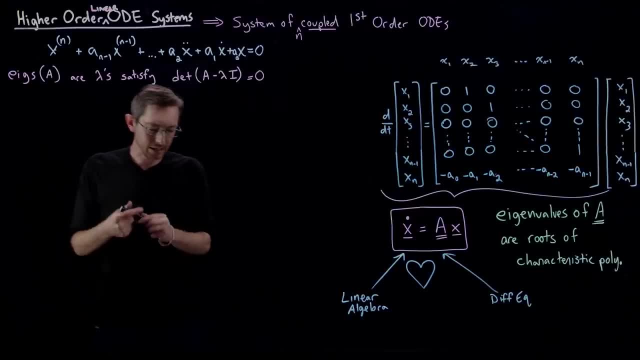 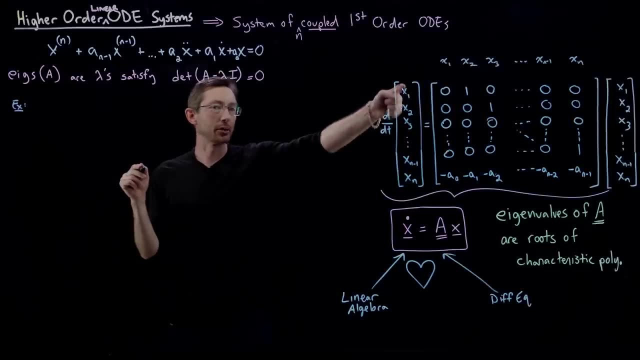 show you on an example. so the example I'm going to do is, let's say, example is: I'm just going to do this up to third order. so I'm going to say I have DDT of X, 1, X, 2, X, 3, and we know that this is going to be 0, 1, 0, 0, 0, 1 and we know that. 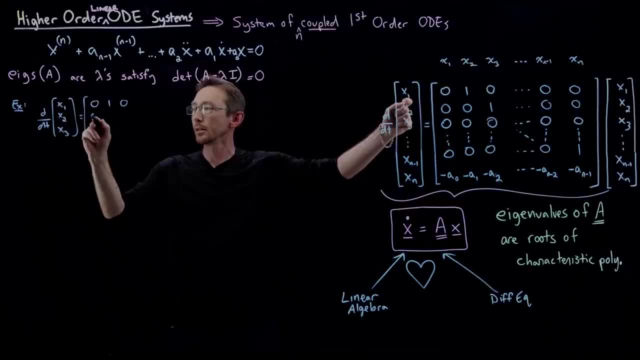 this is going to be 0, 1, 0, 0, 0, 1, and we know that this is going to be 0, 1, 0, 0, 1, and then minus a naught, minus a 1, minus a 2 times X 1, X 2 and X 3, and, of course, 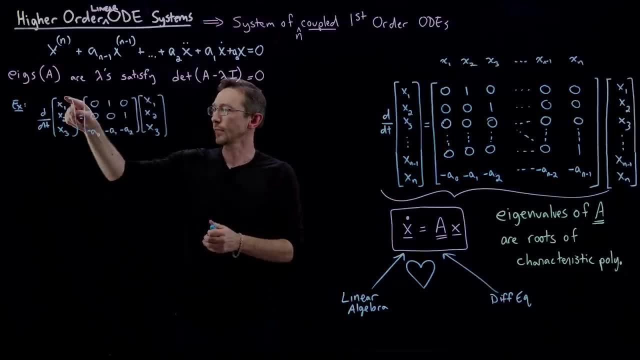 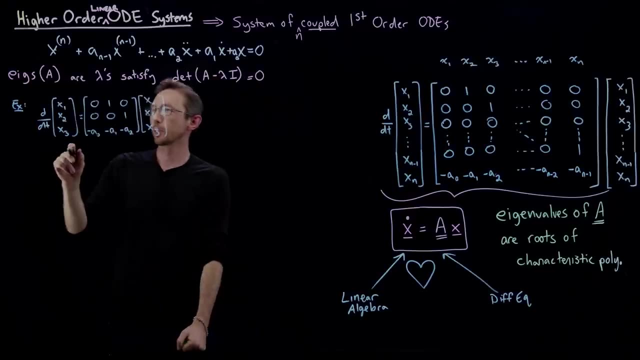 this is the the matrix system representation of a third-order ODE that I'll write out here. so this third-order ODE would be X, triple dot plus, I guess, a 2 X, double dot plus a 1 X dot plus a 0 X equals 0, so I hope you. 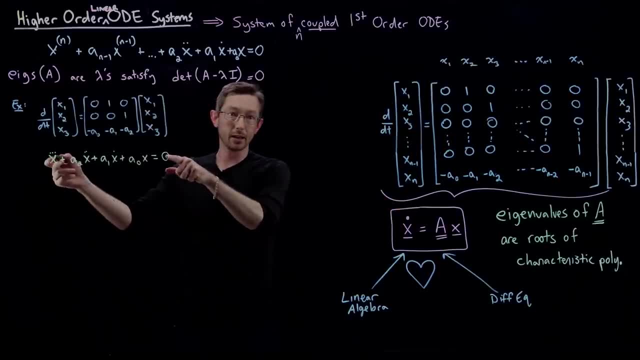 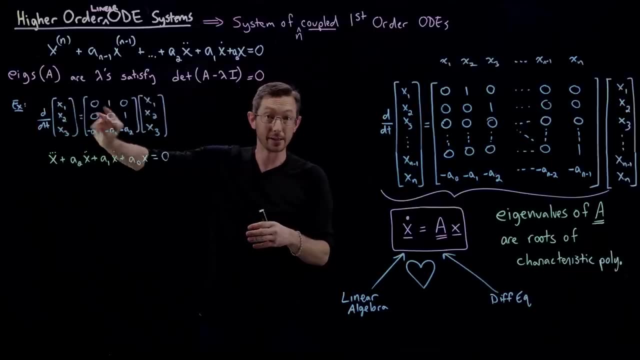 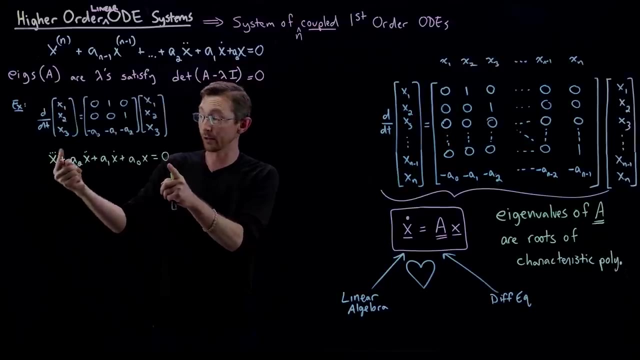 believe and have been convinced that this equation in green and this system in blue are completely equivalent. this is just what happens when you suspend variables and write this as a coupled system of first-order equations, and so I claim that the characteristic polynomial of this ordinary differential equation 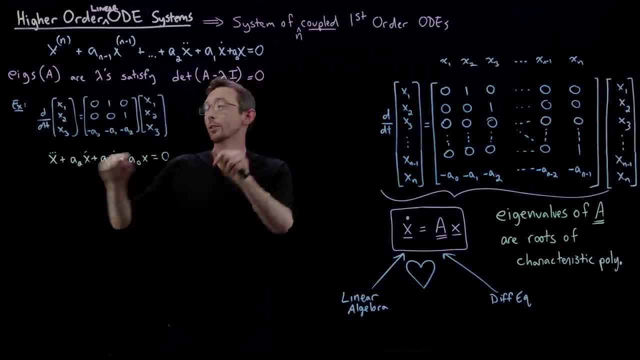 of third order is the same as the differential equation of first-order equations, and so I claim that the characteristic polynomial of this ordinary differential equation as the eigenvalue equation for this system, the equivalent system of first order. okay, and so I'm actually going to take this blue equation and I'm 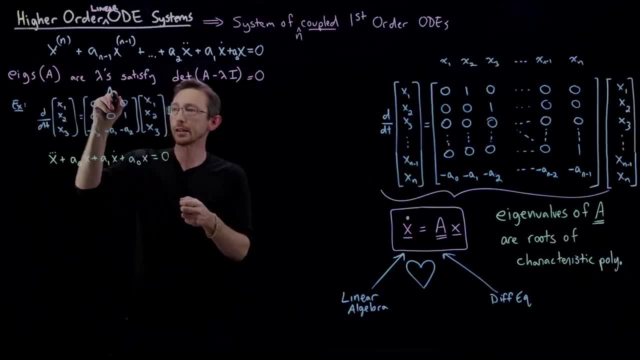 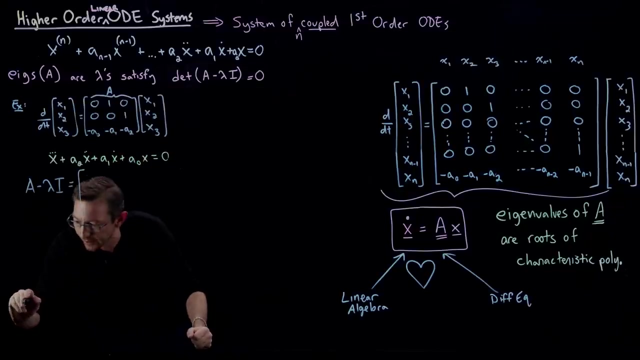 literally going to compute: this is my a matrix here, this, this thing. here is my a matrix. so I'm literally going to compute a minus lambda i, a minus lambda times the identity matrix is this matrix, literally this matrix minus this. an identity matrix just has diagonals of one. so maybe I'll write down here: you know, lambda i. 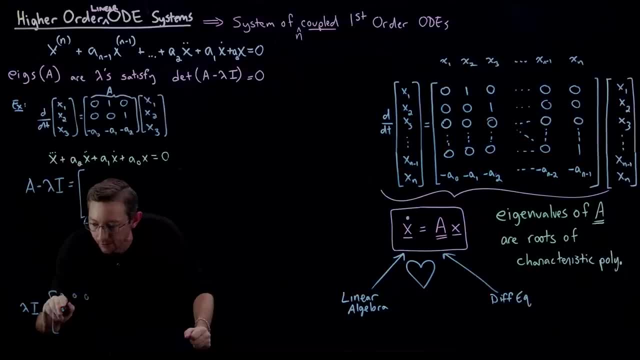 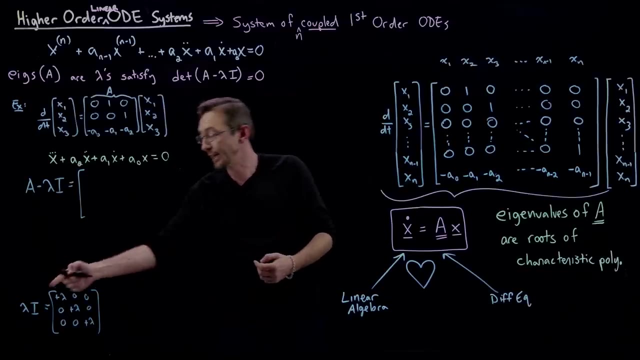 equals minus lambda: zero, zero, zero minus lambda, zero, zero, zero minus lambda. it's literally a diagonal matrix of of plus lambdas. these are plus just a diagonal man matrix of lambdas because the identity matrix is diagonal of ones. if I multiply it by a constant lambda, it's diagonal. 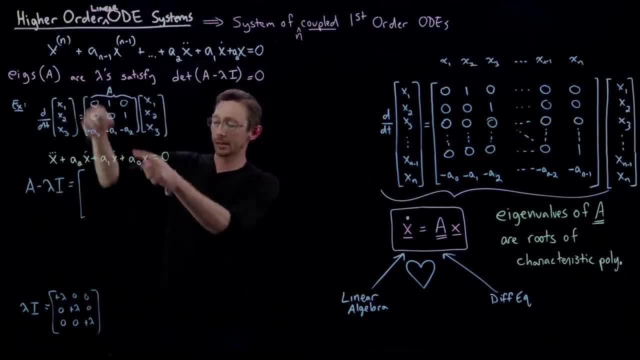 of lambdas. so a minus lambda i is this a matrix minus this matrix, and so that's minus lambda one, zero zero minus lambda. one minus a zero minus a one. minus lambda minus a two. okay, that's not too bad, and now I need to take the determinant of this kind of ugly. 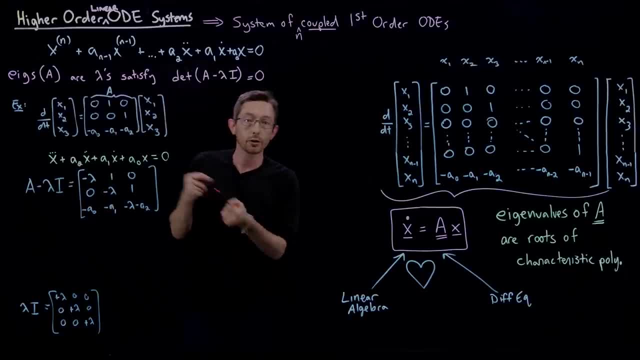 equation and I'm going to take the determinant of this kind of ugly equation and I'm going to expression here. Maybe I'll switch colors to orange just to keep things interesting. So the determinant of A minus lambda- I Now computing, the determinant of a big matrix, is: 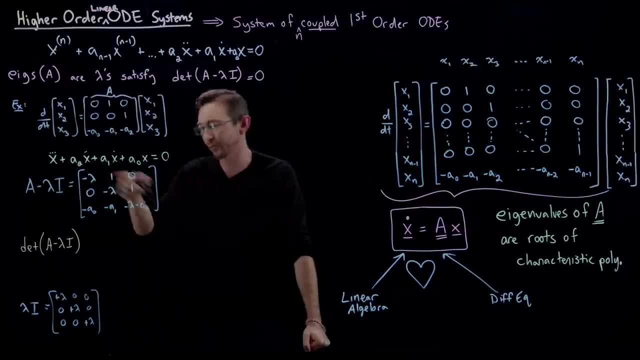 kind of nasty. It's like a combinatorially complex calculation but for a three by three matrix it's easy. I'm hoping you remember from you know high school that it's basically this term times this element times the determinant of this little two by two subblock minus this element times the 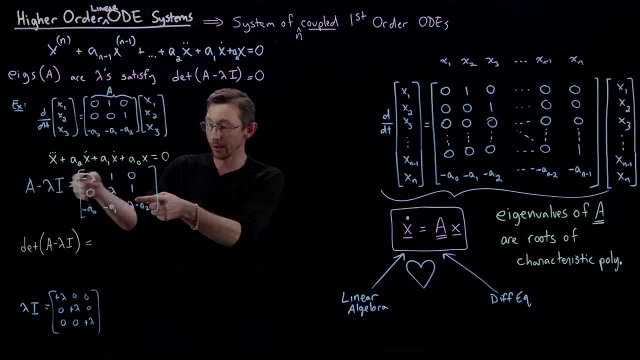 determinant of the two by two subblock, omitting that row and column, plus, this element times the determinant of this little two by two subblock. So we can do this easily: It's minus lambda times this determinant, which is lambda squared plus A2, lambda minus. 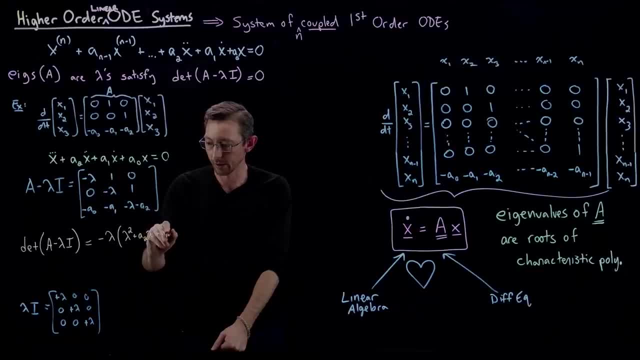 minus lambda, Minus A1, which is plus A1.. I'm really hoping I don't botch this. Okay, that's the first term, Minus one times the determinant of this two by two subblock. So these two multiplied together. 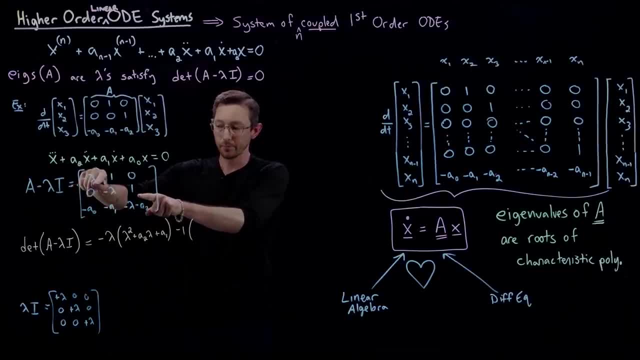 minus. these two multiplied together and that's plus zero. minus minus A0 is plus A0. And then we also have to add zero Times, the determinant of this subblock, but that's just zero. So plus zero. Okay, so that's all the terms for the. 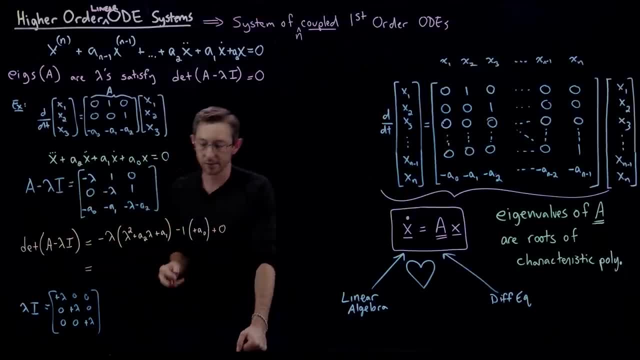 determinant. And if I didn't mess up, that equals everything has a minus sign. So I'm just going to say minus lambda cubed plus A2 lambda squared plus A1 lambda- I already pulled the minus out, So plus A0.. 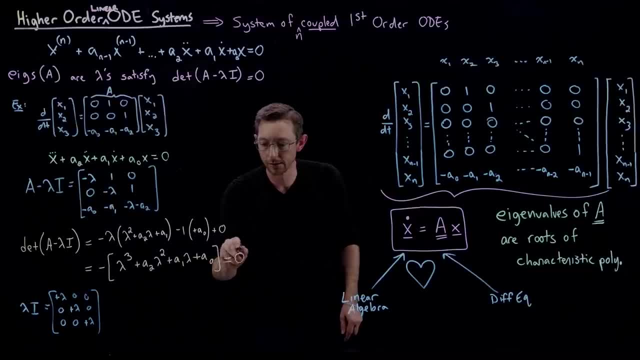 All of that And this determinant has to equal zero. That's the condition Determinant of A minus lambda. I has to equal zero for lambda to be an eigenvalue of A. So this is literally the equation for lambdas that are eigenvalues of this A matrix. But you'll notice that this is also exactly the 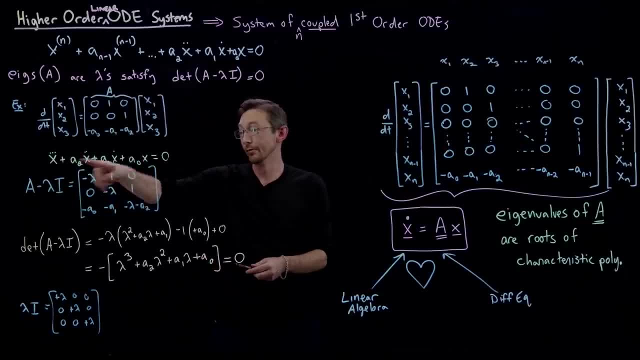 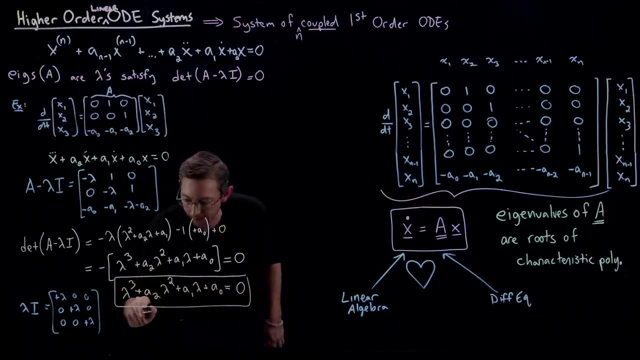 equation for the characteristic polynomial of this differential equation. I'll just write it out: Lambda cubed plus A2. lambda squared Plus A1. lambda plus A0 equals zero. So this is the eigenvalue equation. The eigenvalue equation for A. 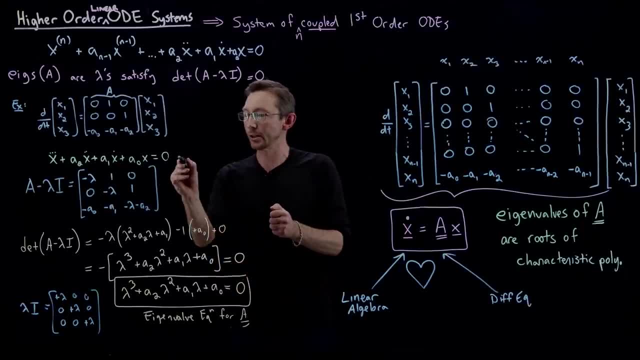 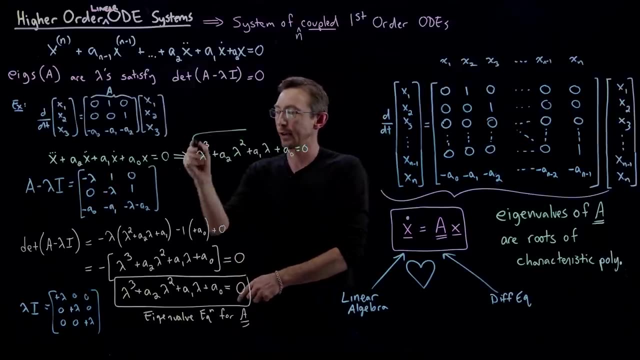 And the characteristic polynomial for this differential equation is, very similarly, Lambda, cubed plus- you can read it off- plus A2, lambda squared Plus A1, lambda Plus A0 equals zero. This is the characteristic polynomial, Characteristic poly And of course, these two are completely equal to each other. 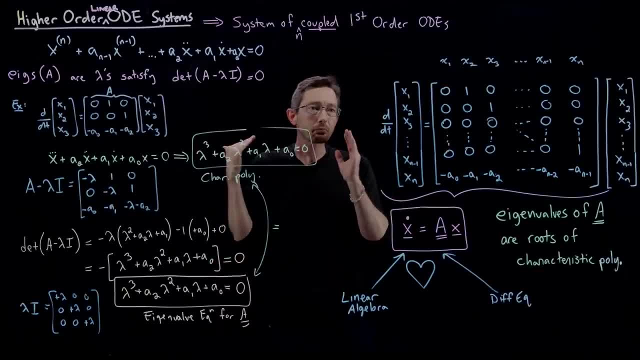 So that's what I wanted to show you is that, yes, in fact, The roots of the characteristic polynomial are in fact, eigenvalues of this matrix A. I can find the eigenvalues of A, and that gives me the roots of my characteristic polynomial. I can find the roots of my characteristic polynomial. 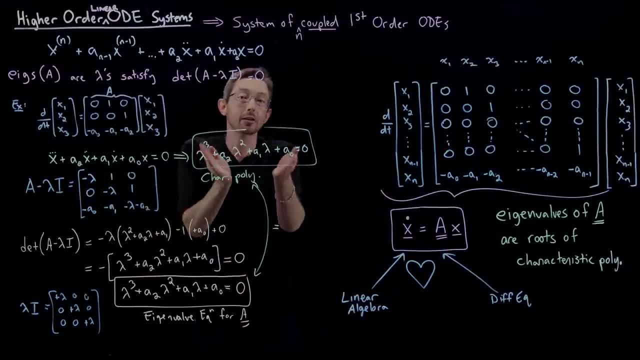 Those will give me the eigenvalues of A. And of course we know that this characteristic polynomial is useful Because it tells me specifically the lambdas that give me admissible solutions. X of t equals e to the lambda t, So that's going to be a solution of this differential equation. 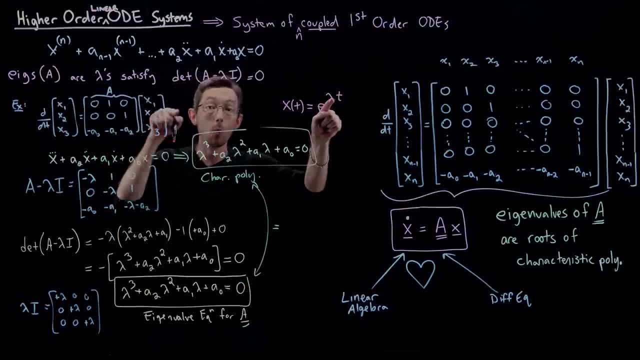 If lambda satisfies this characteristic polynomial or if lambda is an eigenvalue of my A matrix. Very, very useful, Very, very simple. So we're going to come back in force. looking at this system of equations: What are the eigenvalues of A? What are the eigenvectors of A mean? 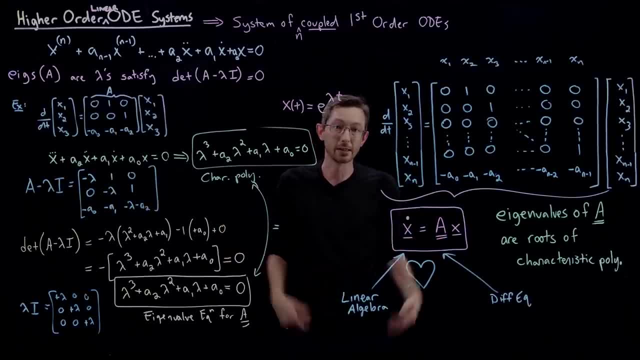 How do we compute them? How do we solve this system using this math? This is kind of my favorite topic and I'm very excited to walk you through it, So stay tuned for more. Thank you.